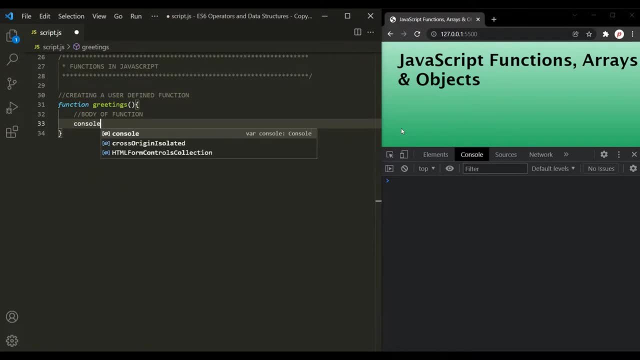 the body of the function. So here let's simply use a consolelog statement And let's log a message in the console saying that: good morning user, welcome back. Okay, so here we have a function with a single line of code. Now, in reality a function can have thousands of lines of code, okay. but here I just want to show you. 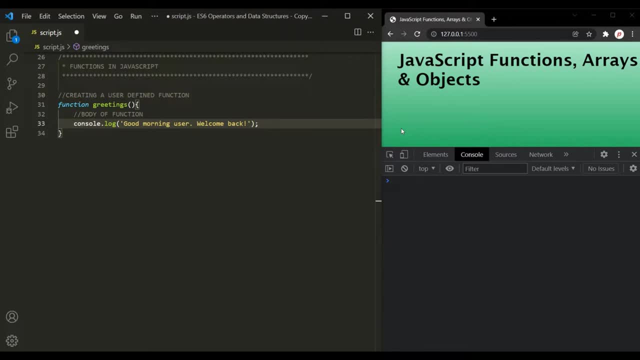 how to create a function. I just want to keep things simple. that's why I have included only one line of code inside this greetings function. Now, here we have simply created a function. It will not get executed unless it is called. For example, if we run this, if this, if we run this code. 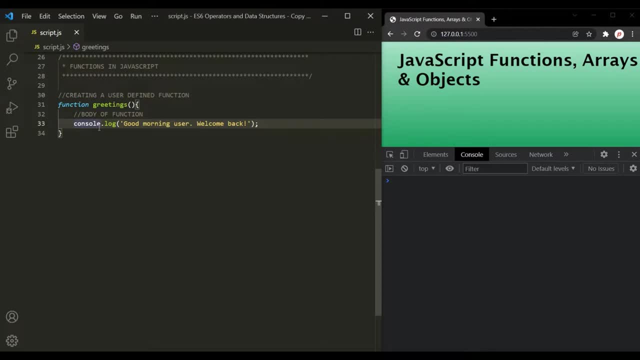 nothing will be logged in the developer console. So if I go ahead and save the changes, you can see that nothing has been logged in the console. In order to execute the body of this greetings, we need to call this function. And to call this function, we can use its name. 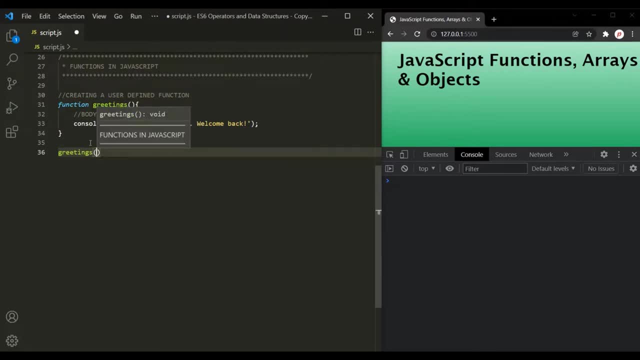 like this, and then on that we can use a set of parenthesis like this. Now, if I go ahead and save the changes, you will notice that the body of this function has been executed and it has logged this message in the console. So, good morning user. welcome back. Now. a function can be called any. 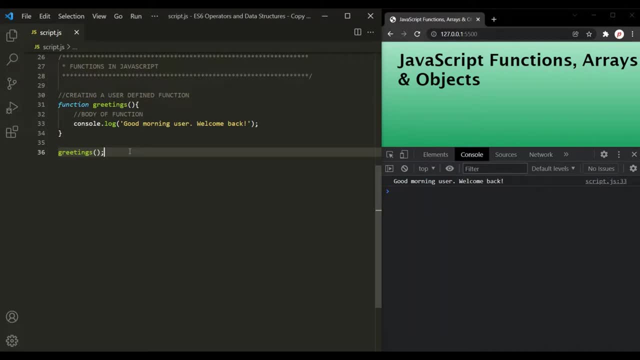 number of times. So let's say I want to call this function. Let's say I want to call this function And every time the function is called, function body will get executed. So here we are calling this greetings function only once, But we can call it as many times as we want. So let's call it two. 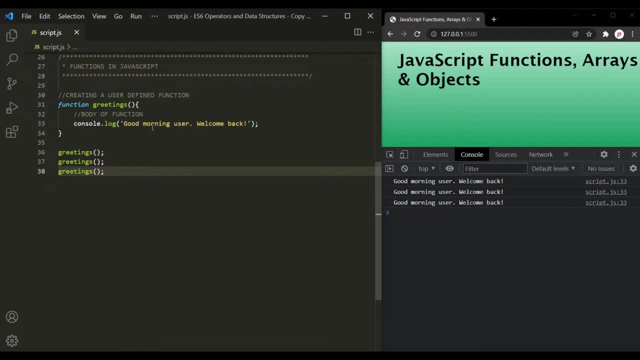 more times And when I go ahead and save the changes, you will notice that the body of this greetings function has been executed three times and it has logged this message in the developer console three times. Okay, and this is how a function helps in writing a code. 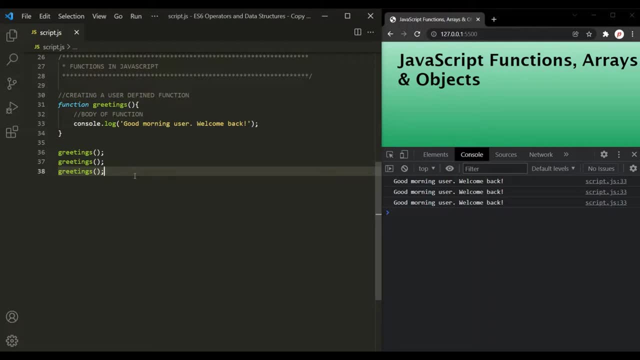 which can be reused again and again without repeating the same code in our program. Now it is also possible to pass some data to the function, and then we can use that data inside the body of the function. and we can pass data to a function using function parameters, and we can. 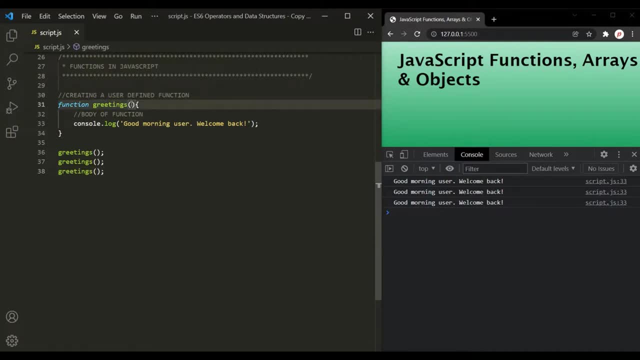 specify the function parameter inside this parenthesis. So let's say, inside this function we want to use the name of the user. So instead of logging good morning user, we want to log the name of the user. So for that here I'm going to specify a parameter and I'm calling it name. 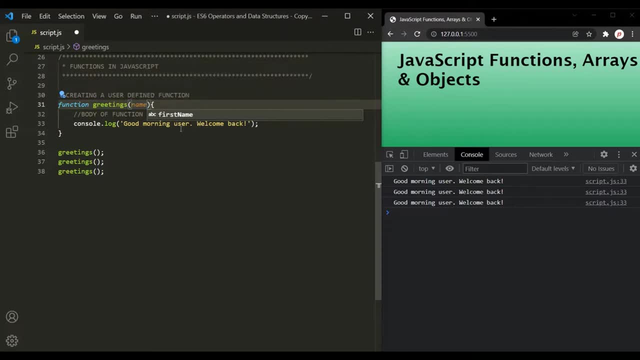 and now I want to use this parameter inside the body of this function. So, instead of logging user here, I want to log the name of the user, like this: Now, from where we will get the value for this name? Well, when we are calling this greetings function, 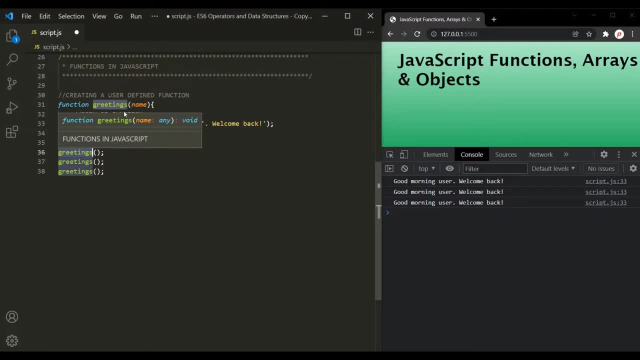 since this greetings function is expecting a value for this name parameter, now we also need to provide the value for this name parameter. So while calling the function, we can specify the value for the parameter. So for the first call, I'm passing John. for the second call, let's pass Mark, and for the third call, let's pass Mary. 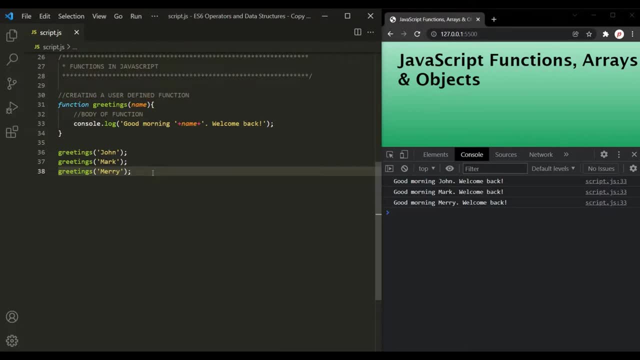 And let's go ahead and let's save the changes. So in the output you will now see that it is logging. good morning John, welcome back. Good morning Mark, welcome back. and good morning Mary, welcome back. So for each call we are passing a value for this name parameter and that value is: 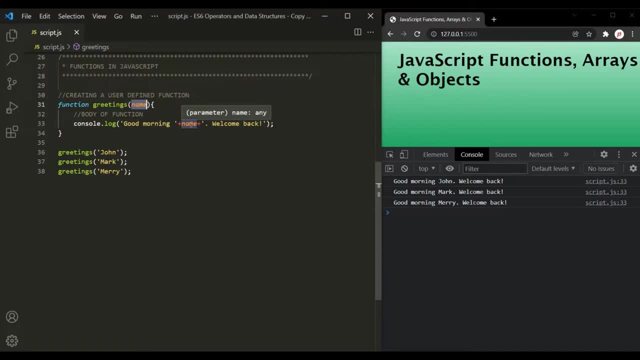 being used in the output. okay, Now, a function can also have more than one parameter. Here we are only specifying one parameter for this greetings function, but we can have more than one parameters for a function and we can specify that by separating the parameters with a comma, like this: so let's say, for this, greetings. 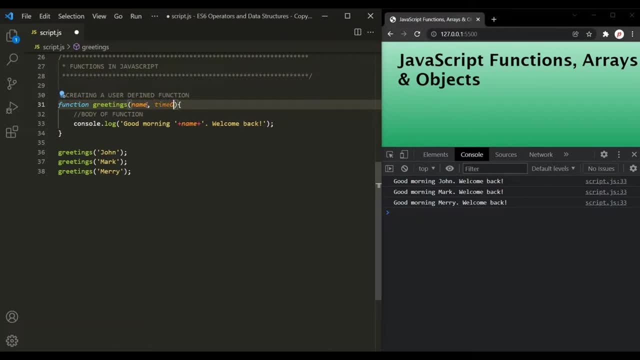 function. i also want to have a time of day parameter, okay, and instead of logging good morning, i want to use this time of day parameter in the output. so again, let's use this time of day parameter here and now. when we are calling this greetings function, we also need to specify the value. 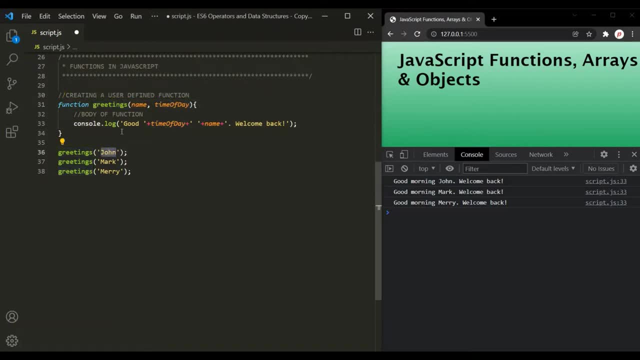 for this time of day parameter. so currently we are passing values only for first parameter, but now we also need to specify the value for second parameter. so for the first call, let's say the value for the time of day is going to be morning. for the second, 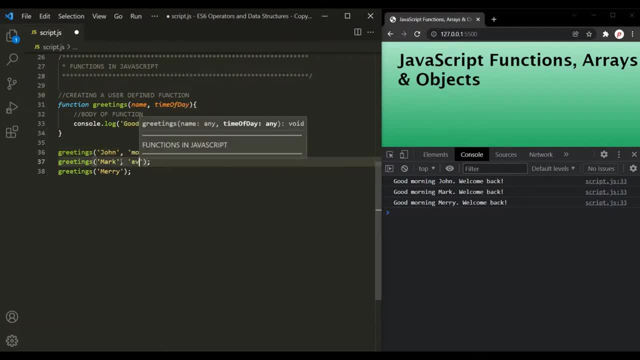 second call, let's say the value for the time of day parameter is going to be evening, and for the third call, let's say it is going to be maybe afternoon. okay, now if i go ahead and save the changes, you will notice that these values are now being used in the output. so good morning, john. 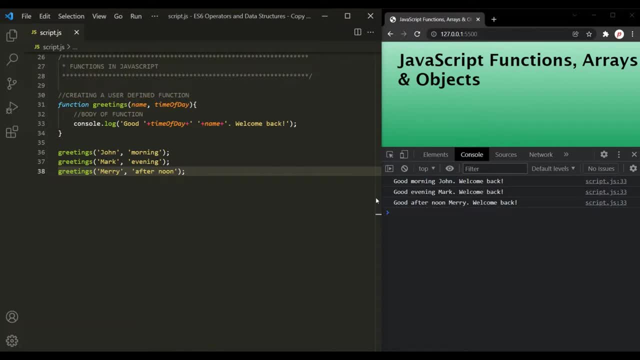 welcome back. good evening, mark, welcome back. and good afternoon, mary, welcome back. okay, so this is how we can pass an input to a function using function parameters. now, one thing which you need to remember here is that when we are specifying these parameters, while defining the function, these values, i mean these variable names- you can say these are called as function. 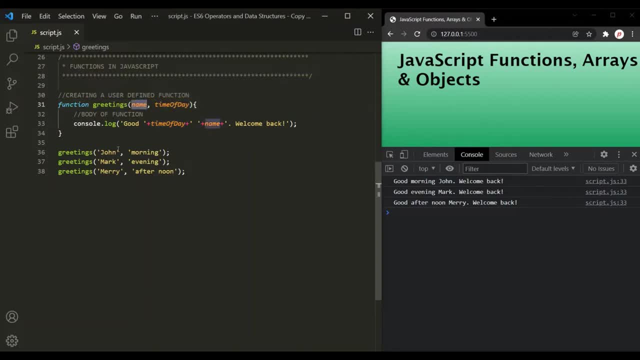 parameters and when we are passing the values for these function parameters while calling the function, these are called as function arguments. okay, so here we are defining this greetings function and we are specifying some parameter list. so these values, you know, these are called as function parameters. and when we are calling 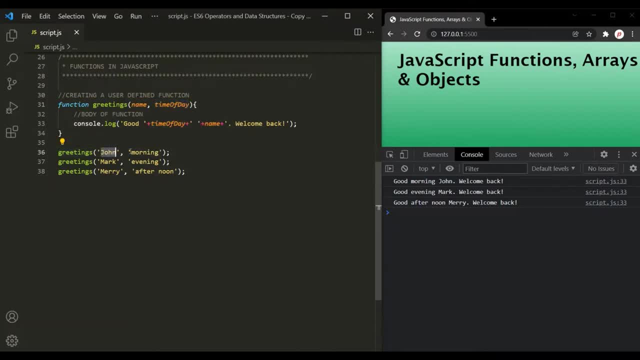 the function. we are passing the function argument. so this john and this morning is the function argument. in the same way, for the second call, this mark and this evening is the function argument, and for the third call, mary and afternoon is the function argument. finally, a function can. 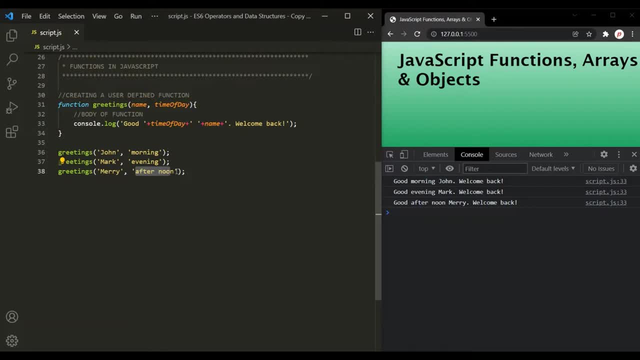 also return a value back to the calling code, and this value can then be assigned to another variable. so let's go ahead and let's create another function. so to create a function, we use function keyword followed by the name of the function. so let's call this function. 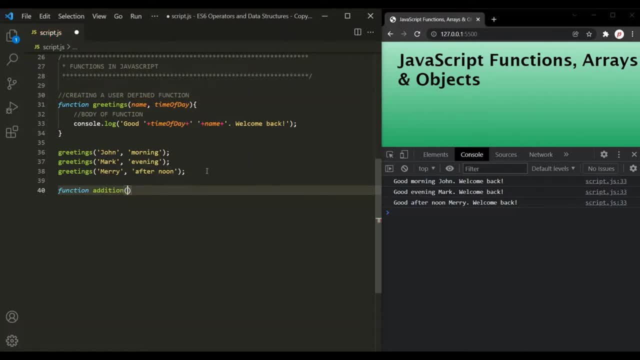 addition, and this function is going to take two parameters. let's call these parameters int one and int two. now, from this function, we want to return the sum of int one and int two, so let's say in one plus in two, and to return a value we use. 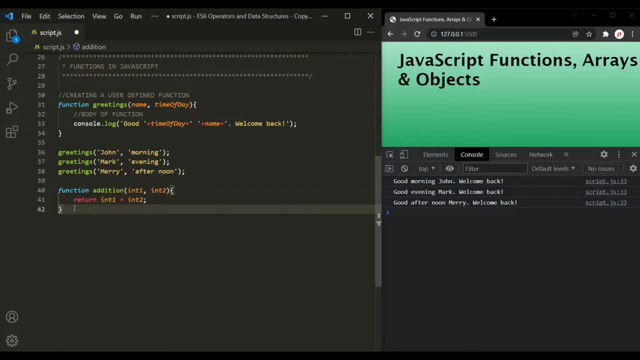 return keyword. ok, now when i go ahead and call this function, this addition function, this function will return a value. so here for the parameters for int one and end. let's pass 20 and 30.. Now, when we are calling this addition function, it is going to pass 20. 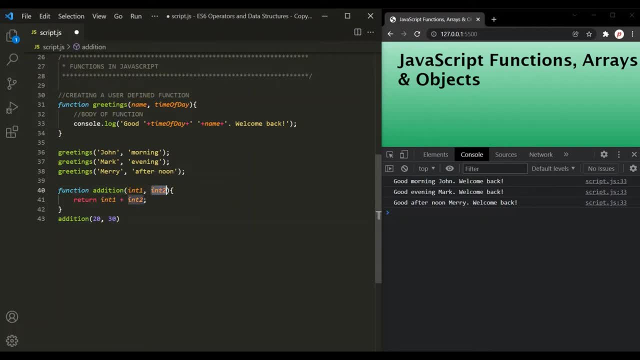 to this int1 and it is going to pass 30 to this int2 and this function will get executed and the sum of int1 and int2 will be calculated and that will be returned from this addition function and we can store that returned value in a variable. So let's call this variable sum. 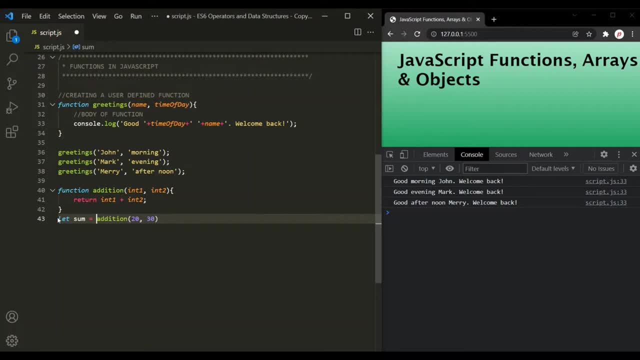 Okay, so now this sum is storing the value which this addition function has returned and what it has returned. It has returned the sum of int1 and int2, that means the sum of 20 and 30. So we can go ahead and we can log this sum variable in the developer console to see the result, If I save. 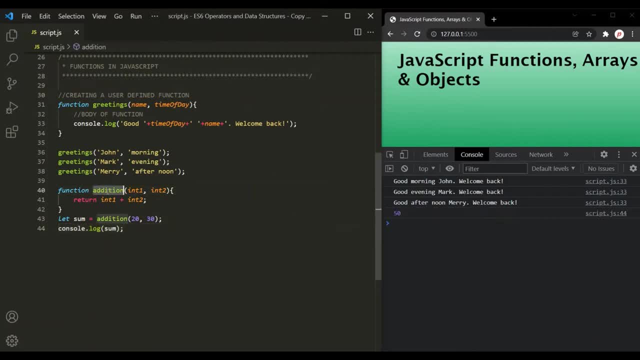 the changes you can see. 50 has been logged. So this addition function returned 50 that we assigned to this sum variable, and now, when we are logging this sum variable, it is logging 50.. Okay, so in this way we can also return a value from a function. Let's call this: 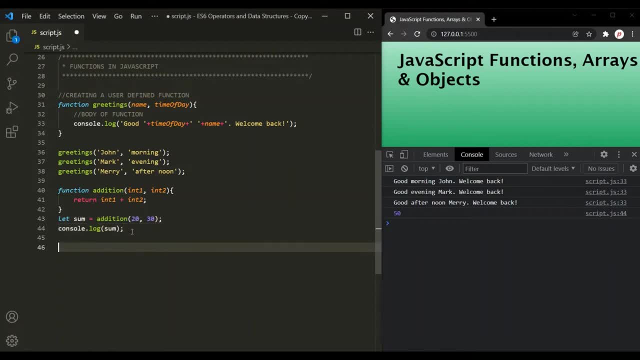 addition function one more time, and this time let's pass some other values. So let's say 120 and maybe 300.. So this time this addition function will add these two numbers and it will return the result. Let's store it in another variable, Let's call it someone, and now let's go ahead and save the. 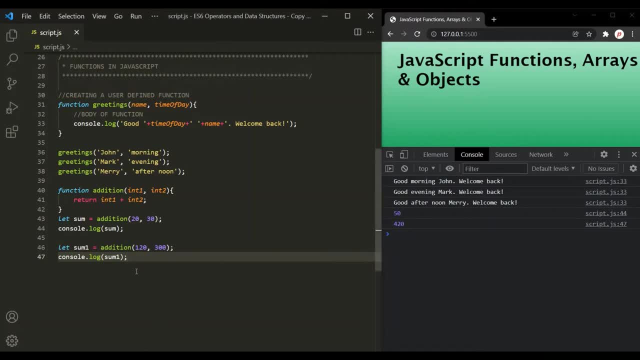 changes. Okay, so now it has logged 420.. So in this way, this addition function is returning some value. Now, one thing which you need to remember here is that when you use return keyword in a function, when javascript engine encounters this return keyword, it will immediately exit that. 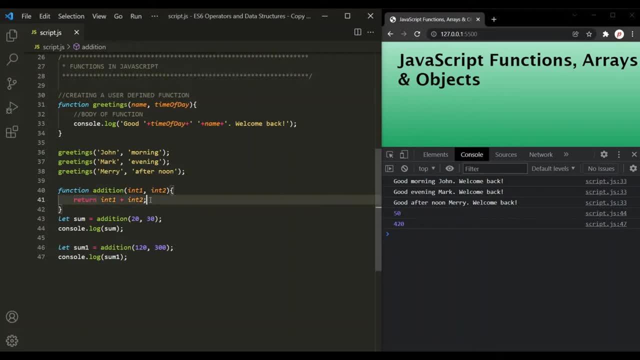 function. Okay, so if there is any other code after this return keyword, let's say we have this consolelog statement and from here let's simply log hello. This line of statement will not get executed because, as soon as you know, when we are calling this addition function, the execution of the body of this addition function. 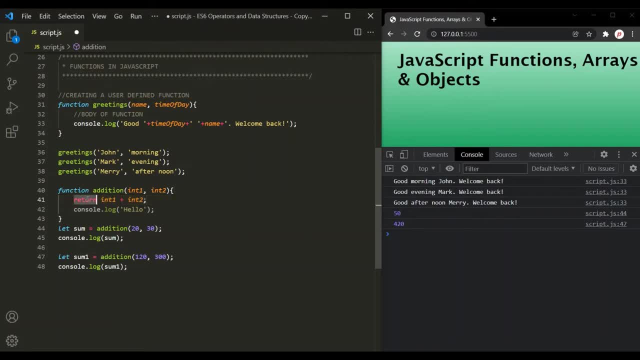 will start and as soon as the javascript engine encounters this return keyword, it will immediately exit the function. So the next line of code will not get executed. and to prove this, let me go ahead and save the changes And you can see that this line has not been executed, because in the console you will not see. 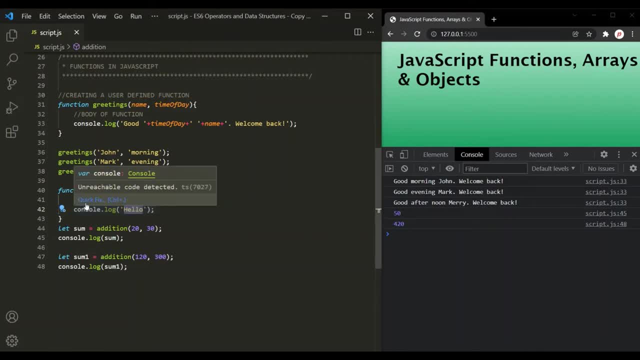 this hello logged anywhere. Okay, so after return keyword, if you have any statement, that will not get executed, because as soon as javascript engine encounters this return keyword, it will exit immediately from the function. Now in a function you can write many return keywords. Let me show. 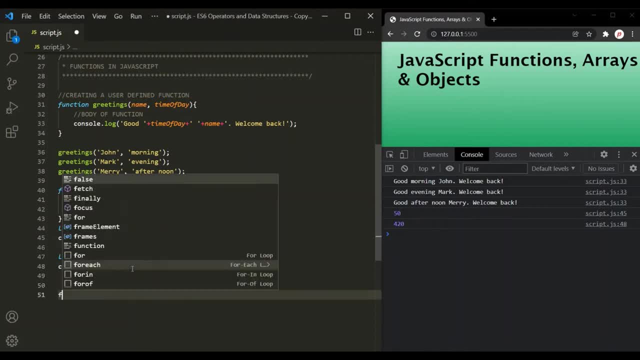 you what I mean by that. So let's create another function, Let's call it isEligible or let's call it isEligibleForVoting, Okay, and to this we will pass a age-parameter. Now, inside this function, I want to check if age, if it is. 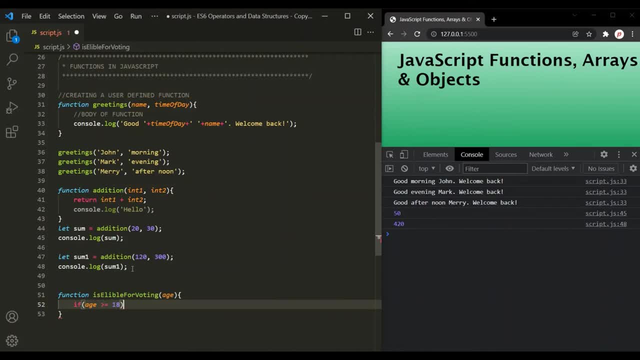 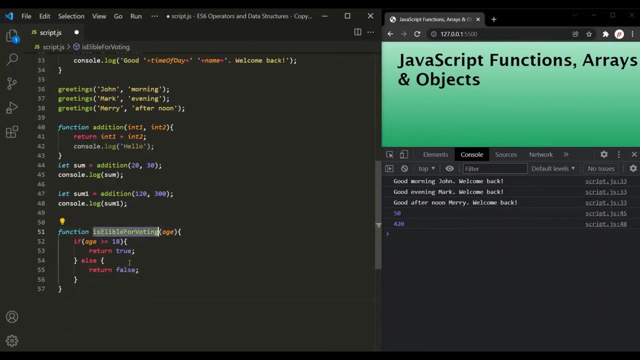 greater than or equal to 18, then I want to return true. So here can say return true. Else, if age is not greater than or equal to 18, then i want to return false. so here let's say return false. okay, so in this function this is eligible for voting function. you can see we have two. 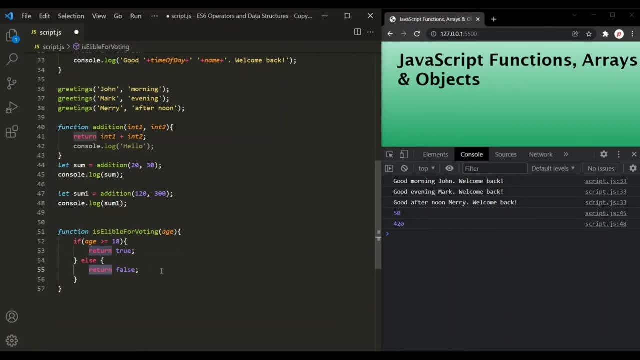 occurrences of return keyword. now, whichever return keyword will be encountered first, that value will be returned and the function will exit immediately. so let's call: this is eligible for voting and here let's pass 30. now, when we are calling this is eligible for voting, this function will be called. age will be assigned with this value, 30, and inside the function we are. 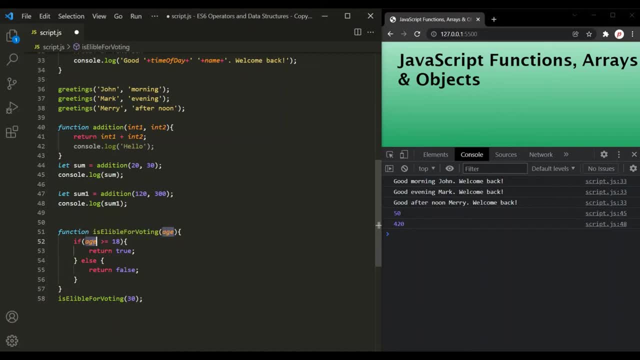 checking if age is greater than or equal to 18. now, 30 is clearly greater than 18, right? so this if statement will return true and this block will be executed and from here, true will be returned okay, and the function will exit immediately. so let me go ahead and log the value returned by. 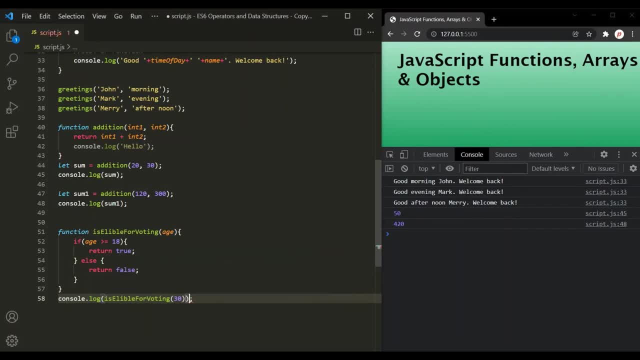 this function in the developer console. if i save the changes, you can see true has been returned. now let's call this function one more time, and this time let's pass 12. so when we are calling, this is eligible for voting and when we are passing 12, this age will be assigned with the. 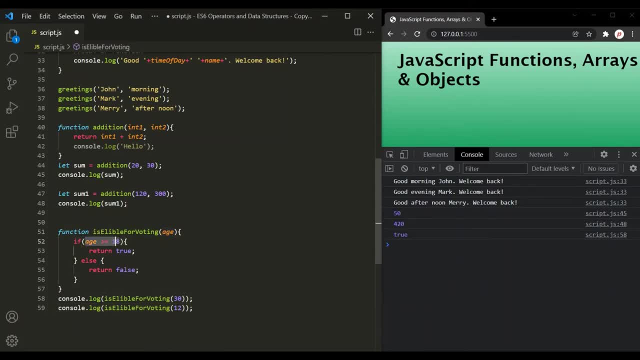 value 12 and again this condition will be checked. now, 12 greater than equal to 18, this condition will return false. so here this else block will be executed and from the else block we are returning false. so here this is eligible for voting will return false. if i save the changes, you can see. 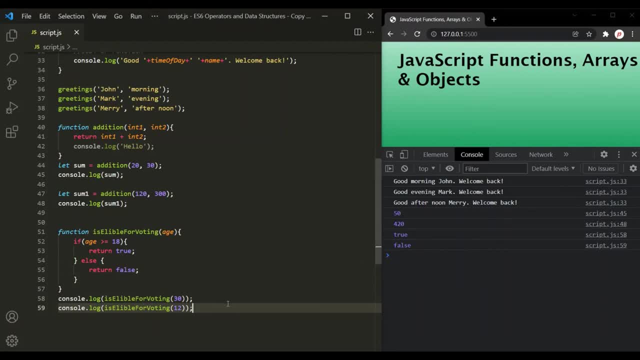 false has been logged here. now we can also use return keyword without returning any value. for example, let's say, here we are calling this is eligible for voting, and if i save the changes here, i use this return keyword, but i am not returning any value. what will happen in that case? 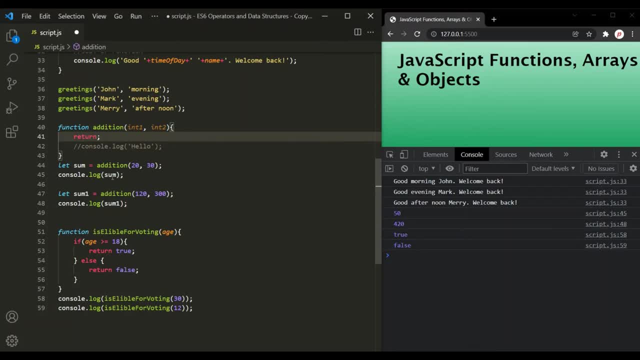 let's see that. so when i save the changes now, currently, when we are calling this addition function, it was returning the sum of int1 and int2, but now we are not returning that value, we are not returning anything from this addition function. so now, if i go ahead and save the changes, 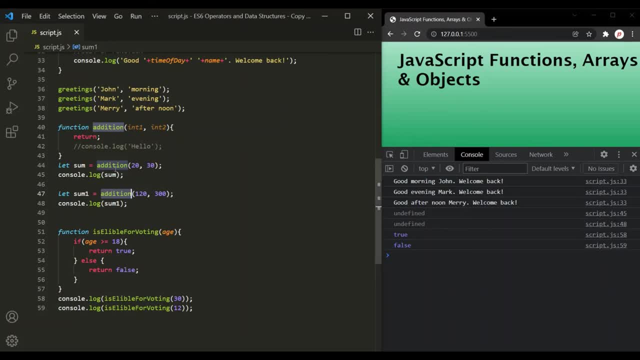 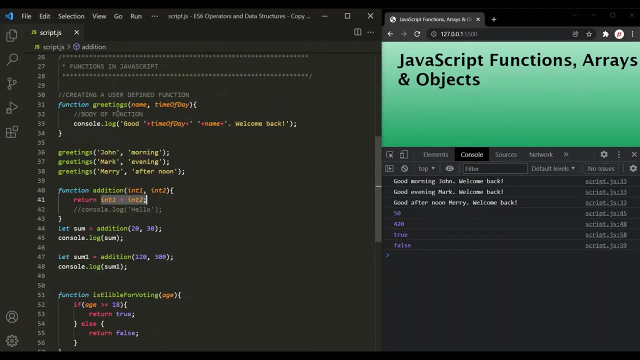 you will see that undefined has been returned from this function. okay, so when we do not return any value from a function, undefined will be returned. so remember this point. now, if i scroll up, in this greetings function, we have not used this return keyword, right? so if i go ahead and assign this, you know the result of this greetings- to this variable x. 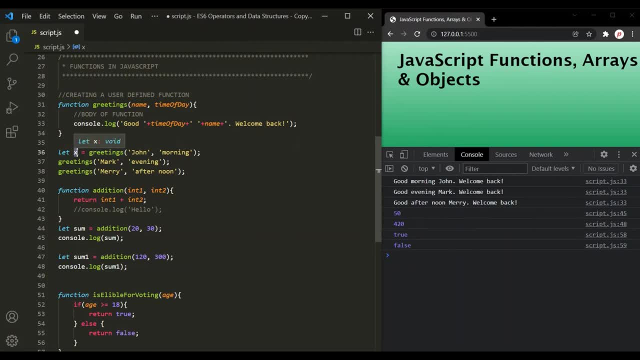 what do you think will be assigned to this variable x? because from this greetings function we are not returning any value, right? so let's see what will be assigned to this x. let's log this x, let's save the changes and you can see: undefined has been logged. so, first of all,